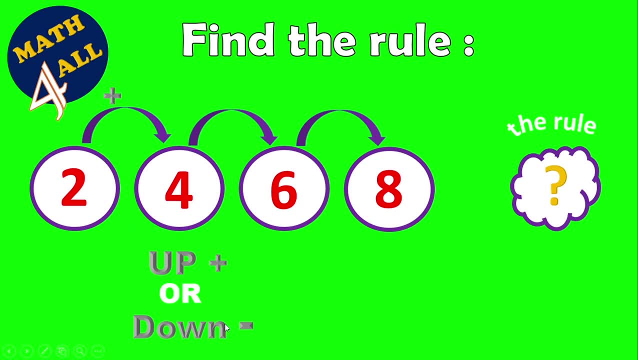 If you are decreasing, you are counting down. so you will put minus sign Here. 2, 4, increasing. so we put plus sign. 4, 6, increasing, you will put plus again. 6, 8, increasing, we will put plus sign again. So the first part in the rule is plus sign. The second part, you will subtract. Let's subtract. 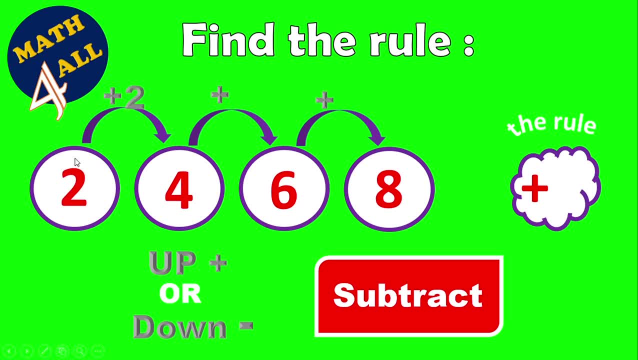 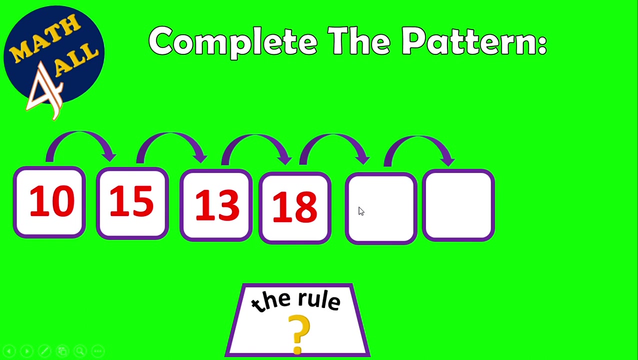 4 minus 2 equals 2, so we add 2.. Here, 6 minus 4 equals 2.. 8 minus 6 equals 2, so this is the pattern Plus 2.. In each step you add 2.. 2,, 4,, 6,, 8.. This is the pattern and this is the rule. The second pattern: Here we have a missing number, so you should find the rule to know this missing number. 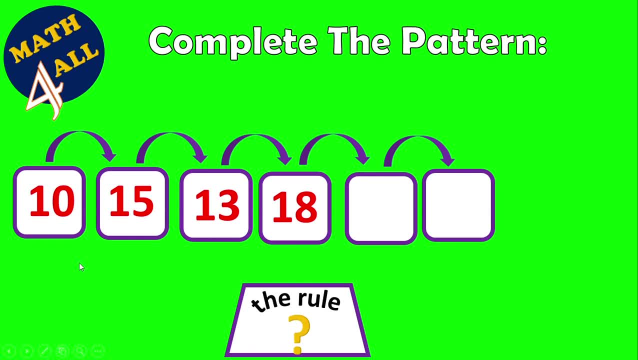 Let's find the rule We said. the first step: ask yourself: we are counting up or down? If you are counting up, we will put plus sign. Let's see 10,, 15, we are increasing, we will put plus sign. Okay. The second step: 15, 13,. you are decreasing. 13 is less than 15, we are decreasing, we are counting down, so you will put minus sign. 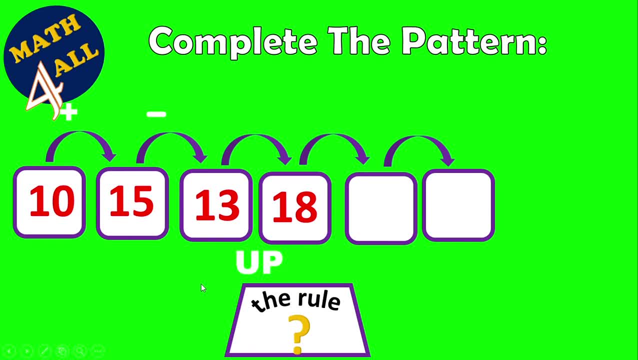 13,, 18, you are increasing again. we are counting up again. Let's put plus sign. So the pattern, the first part, will be: Add, subtract, plus, minus, plus, minus again and then plus. This is the first part In the rule. the second part, you will subtract. 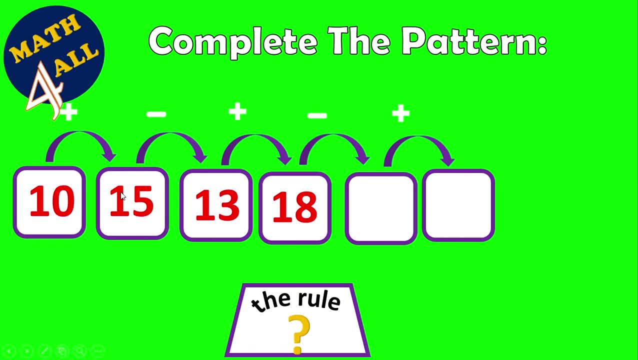 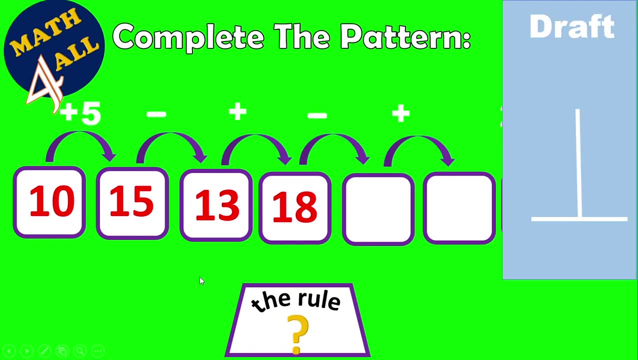 Let's subtract. We will subtract: 15 minus 10 equals 5.. 15 minus 13,. let's subtract: Here we have 10th unit and then 15.. 15 minus 13,. 5 minus 3 equals 2.. 1 minus 1, 0, so it's 2.. 15 minus 13 equals 2..